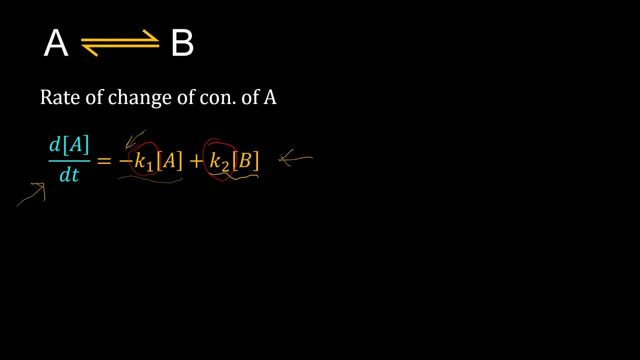 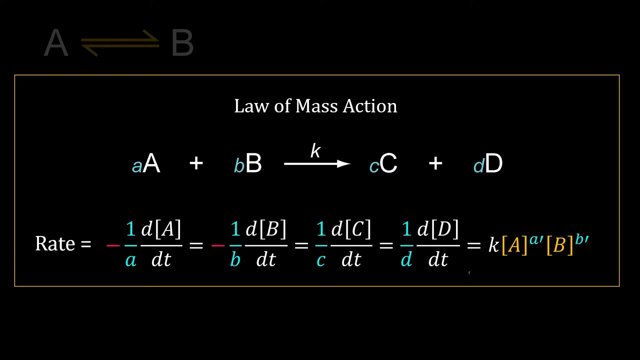 You must have noticed that this ODE is based on the law of mass action. I assume you remember the law of mass action. In brief, the law of mass action says that the rate of a reaction is proportional to the concentrations of the reactants raised to the power of their respective orders. 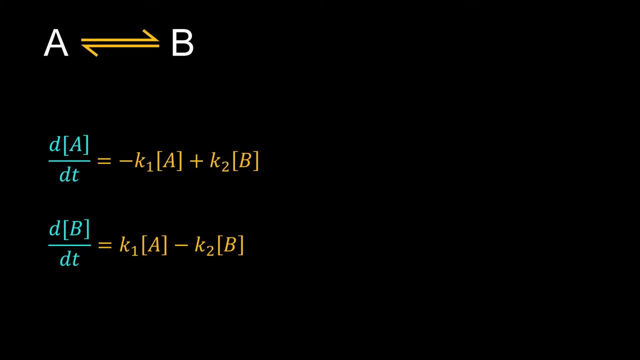 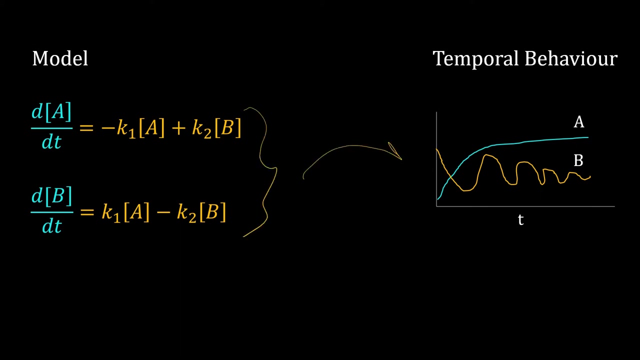 I have written the second ODE. The second ODE represents the rate of change in the concentration of B. Now we have the model with two ODEs, But remember, we want to know the time evolution of A and B. So from the model we have to get the temporal behavior of A and B. 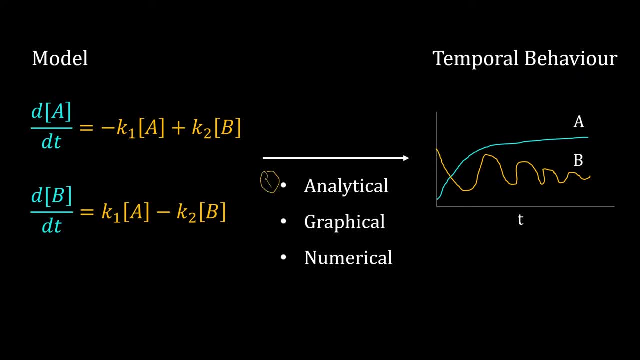 For that we have three approaches. We can solve these ODEs analytically, The way you use to solve difference in values. For that we can take the ODE as the first step. In the second step we have two only. 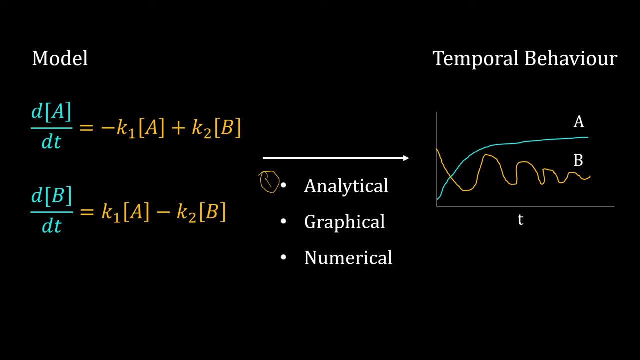 The first step we need to calculate the general problem of the differential equation. We then get the differential equations by paper and pen. otherwise we can also use a graphical method. we will learn the graphical method in another video. in this lecture I will use the third approach: numerical solution of this system of ODEs. I will 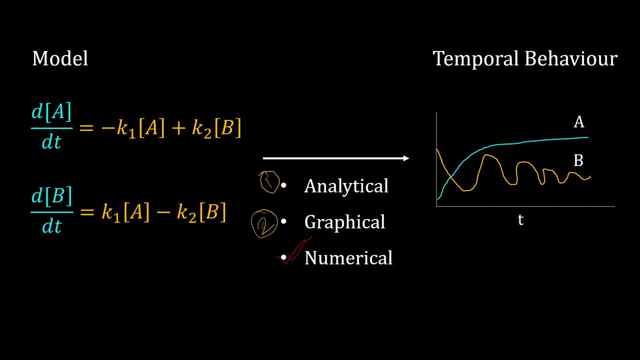 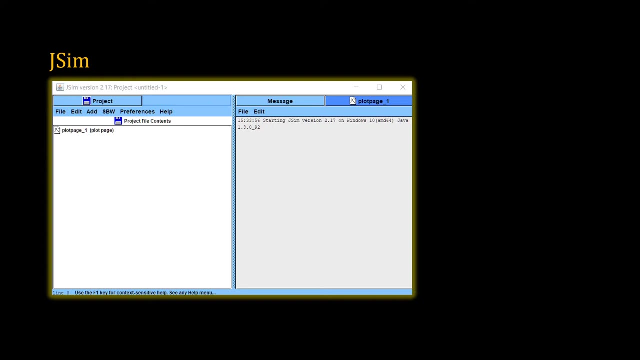 discuss the algorithm for the numerical solution in details in another video for this model. here in this lecture I will use a software and show you the results. I have used a software called Jessing to simulate our model. it is very easy to use. we have a video tutorial on Jessing. there are many other software for. 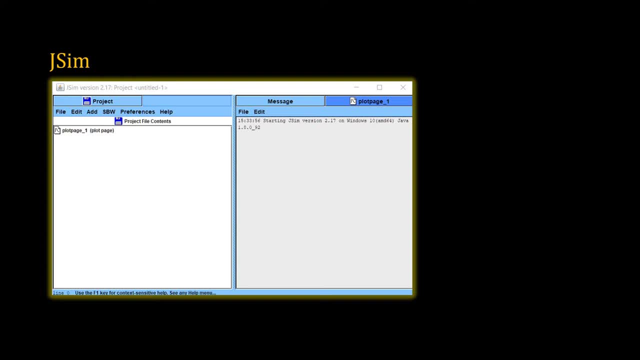 numerical simulation of ODEs models. you can use any of those to solve the model. we must specify the initial condition. I have considered that at t equal to zero, that is, the initial time point is equal to 10 molar and that the initial time point A is equal to ten molar. and 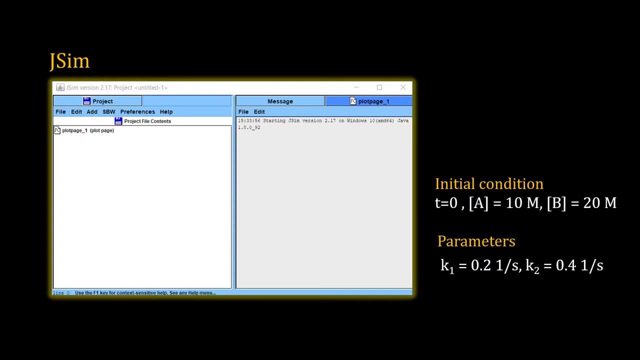 for the initial time point, that is, the initial time point A is equal to 10 molar and that the initial time point A is equal to ten molar and and B is equal to 20 molar. We also need to specify the values of the parameters of the model. 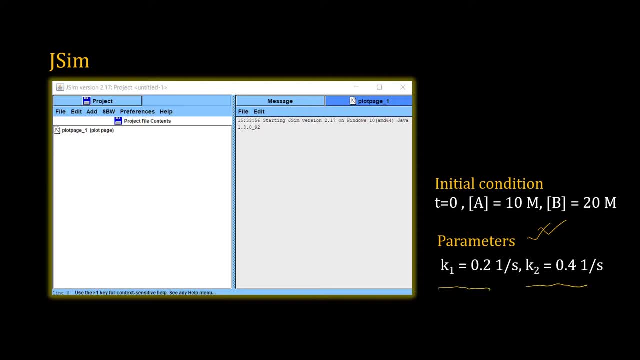 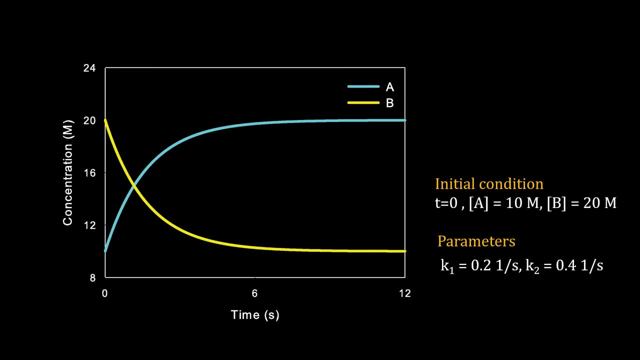 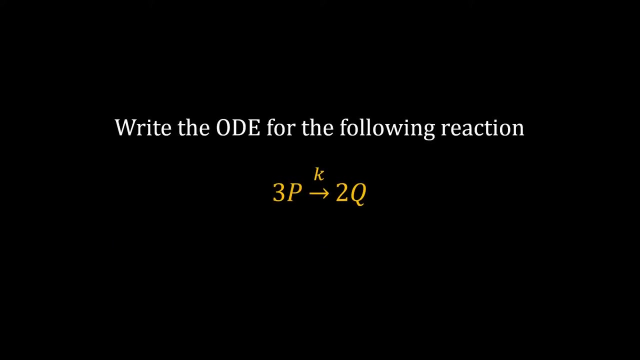 So K1 is equal to 0.2 and K2 is equal to 0.4.. This graph shows the data generated by Jason. With time, A increases but B decreases. eventually both of those flattened. Here is a quick question for you. 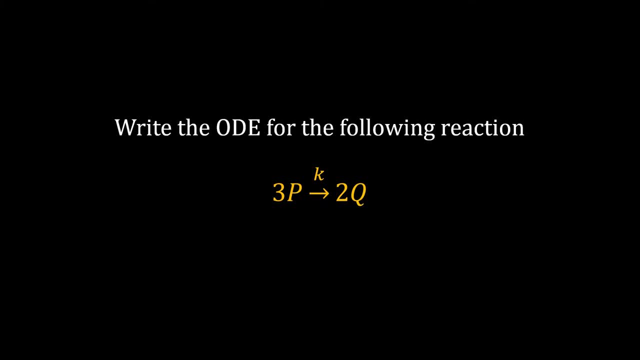 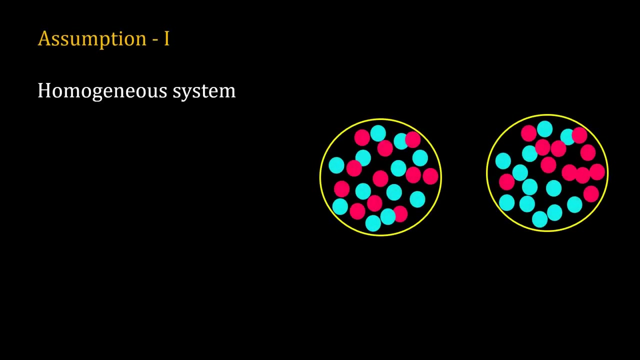 Write the ODE for the rate of this particular equation using the law of mass action. Hope you are done with the problem. Every ODE based model has two assumptions. I will now discuss those assumptions. Our first assumption is that the system is homogeneous. 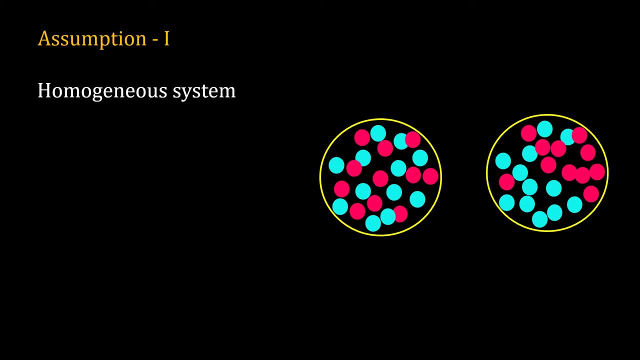 Suppose in a cell we have red colored molecules and blue colored molecules. In this cell all the molecules are well mixed, So the concentration of the molecules does not depend upon the location inside the cell. Our rate equation will have only one independent variable time. 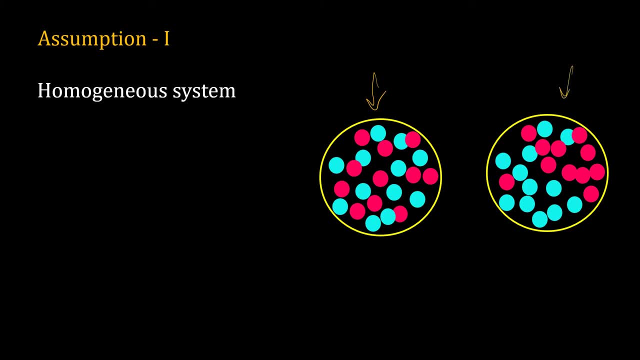 But in the other cell you can easily notice a gradient Rate. molecules are more on the right side. That means the concentration of molecules depends upon the position inside the cell. So the rate of reaction will also depend on location. Therefore here the position is also an independent variable. 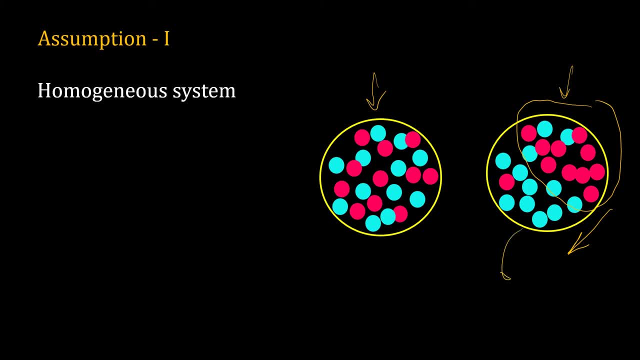 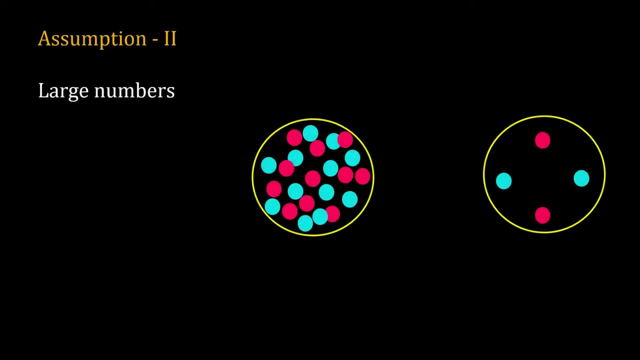 For this system. we cannot use ODE. We have to use partial differential equation. A partial differential equation will have two or more independent variables. The second assumption is that the system size is large. If we are dealing with molecules, then we must have a large number of molecules. 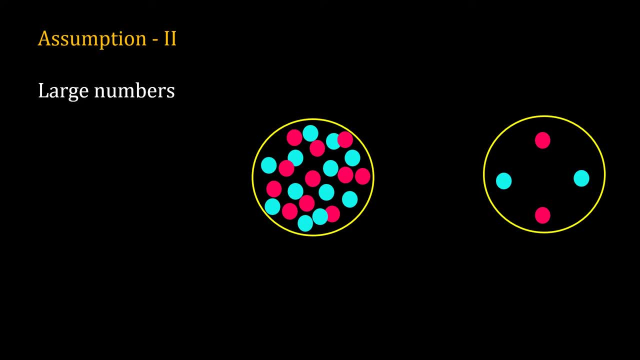 Take the example of red and blue molecules again. Suppose these molecules are reactants of a reaction. When a red molecule hits a blue one, we have a product. On the left-hand side, we have a product. So we have a product. 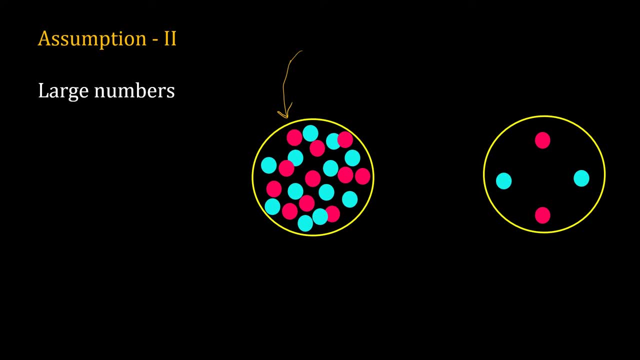 On the right cell we have lots of these molecules. So if we observe this cell almost every other moment, there will be a reaction, So we will get a smooth increase in the product. Now take the other cell. Here we have only a handful of molecules. 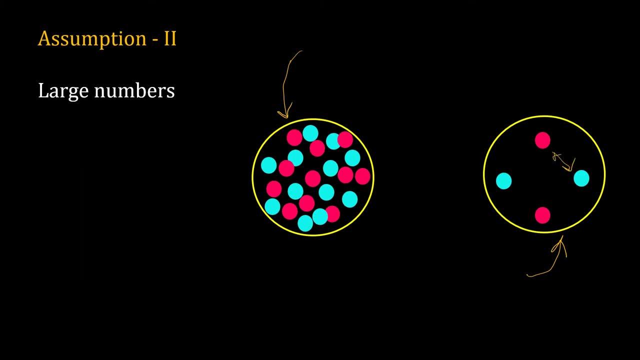 Right now a red molecule may hit a blue one and then we have a product. But the next reaction may not happen immediately. We may have to wait for one hour, One hour or so that one red molecule diffuses close to the blue one and hits it. 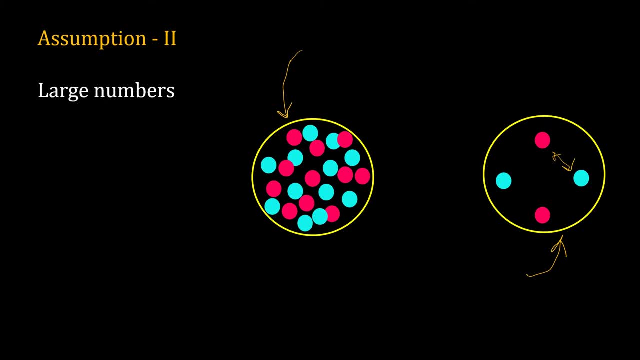 As the number of molecules is low, we are uncertain about the timing of the next event. This type of system is called a stochastic process. A stochastic process has randomness. We cannot use ordinary differential equations to model a stochastic system. Let us try to understand this assumption from another perspective. 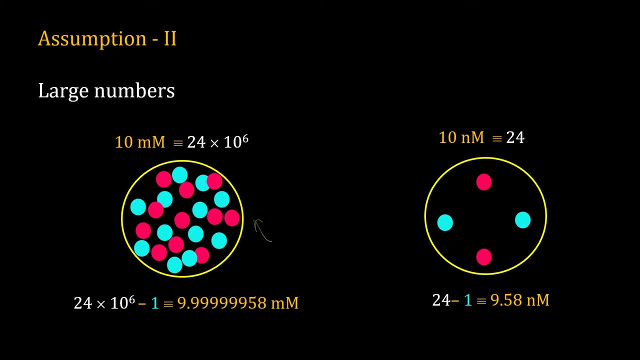 We have a cell of 1 micron size. The concentration of the red molecule is 10 millimolar Approximately. that is equivalent to 24 into 10, to the power 6 molecules inside the cell. Now, when a reaction happens, one red molecule is consumed. 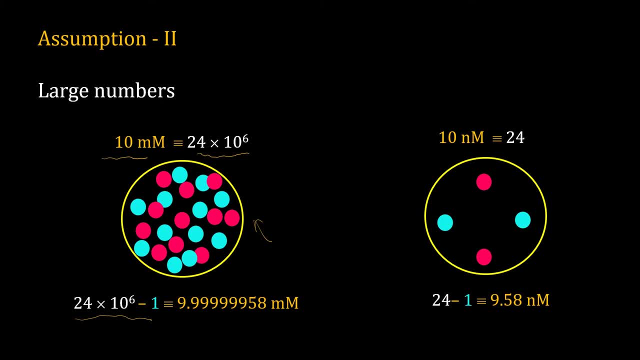 So the number of red molecules decreases. That changes the concentration of the molecule to 9.99999958 millimolar. Hope I am not making any mistake in the number of 9s. Anyway, this change from 10 millimolar to 9.99999958 is very small. 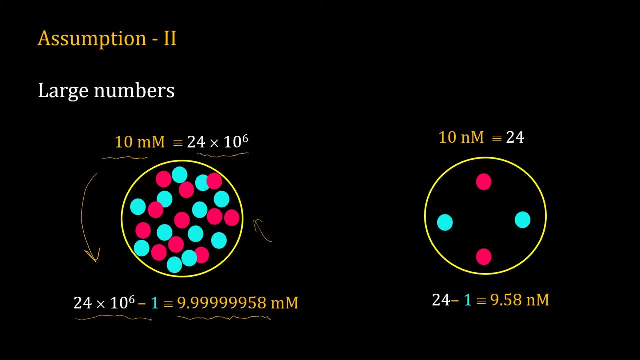 So the concentration of the red molecule is 10 millimolar. So the concentration of the red molecule is 10 millimolar. So the concentration of the red molecule is 10 millimolar And can be considered as a smooth change. 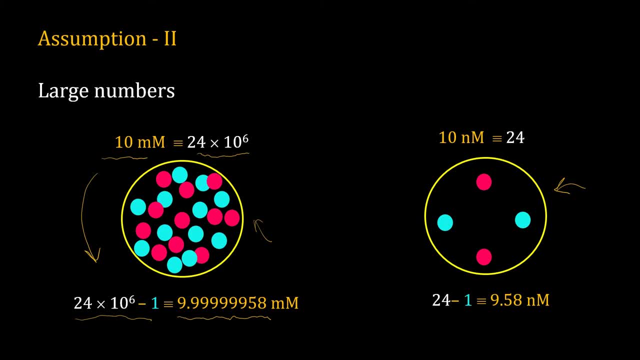 Now take the other cell. Here the system size is small. The concentration of the red molecule is only 10 nanomolar. Using Avogadro number, approximately that is equal to 24 molecule. When a reaction happens, the number changes by 1.. 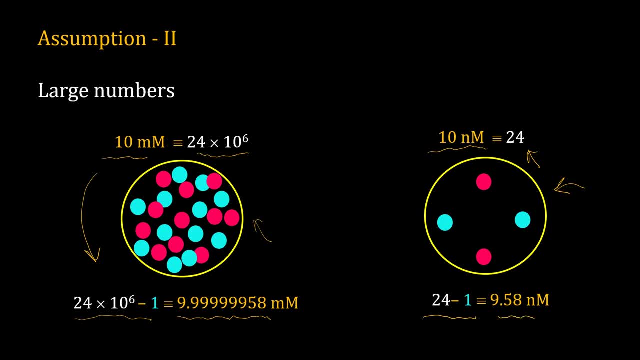 And the concentration drops to 9.58 nanomolar. Numerically that is an average. I hope you remember that we can use a differential equation only when the variables are changing smoothly. So for this cell with a low number of molecules we cannot use ODEs. 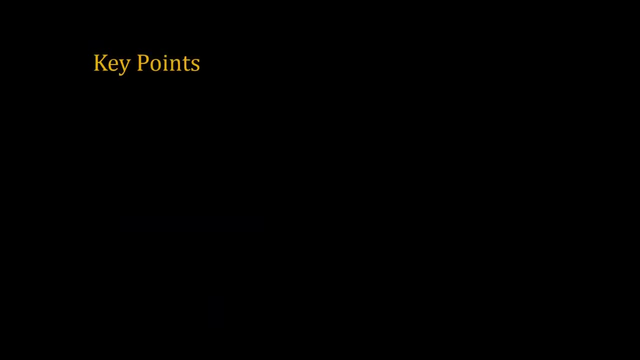 Let's jot down the key points of this video. By dynamical modeling, we capture the time evolution of a system. In differential equation based models, we use ordinary differential equations to represent rates of processes. Once we have the model, we can explore the temporal evolution of the system using three 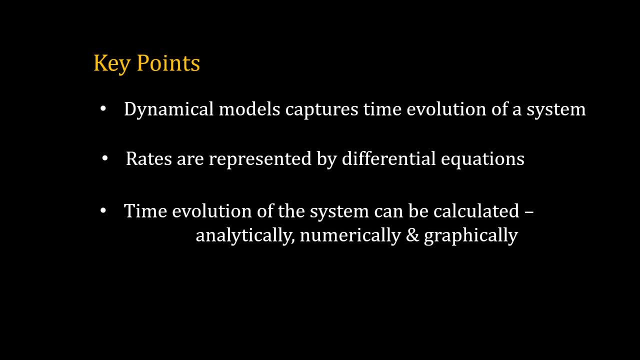 methods: Analytical method, graphical method and numerical method. And the final point: We have two assumptions behind every ODE based model: The system is homogeneous or well mixed And the system is large. The number of molecules in the system is large. 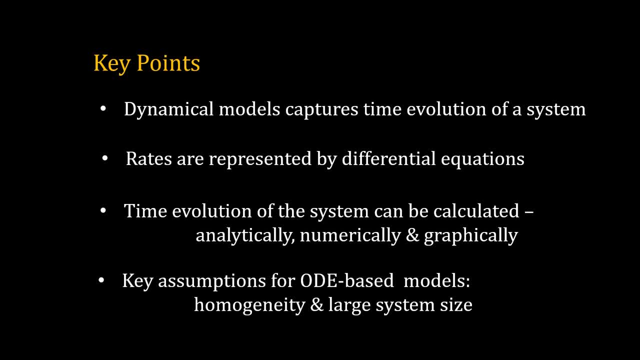 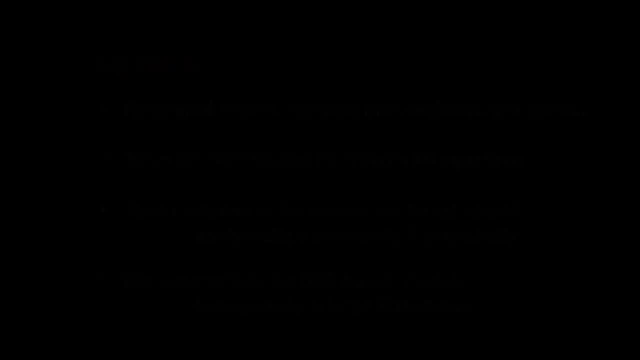 The number of molecules in the system is small. The number of molecules or the number of components in the system is very high And the occasional level of Pearl-Halkvale and De. 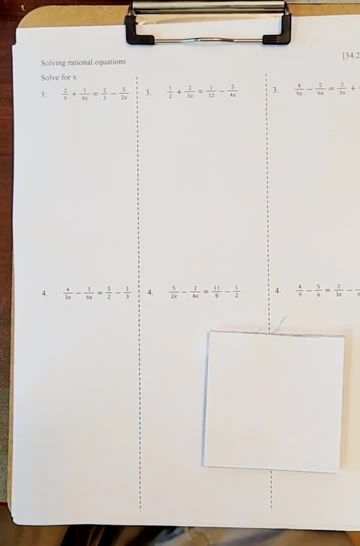 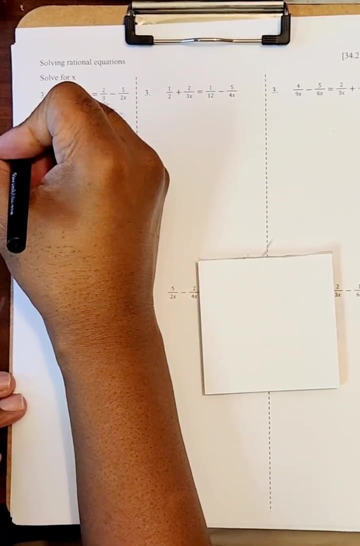 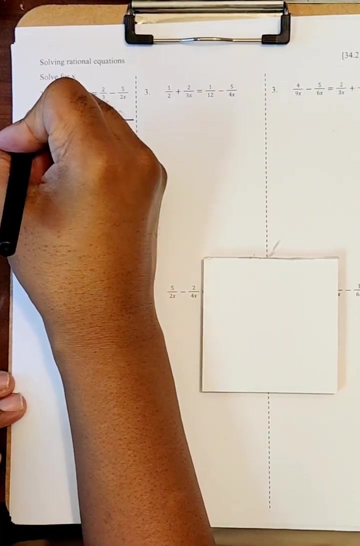 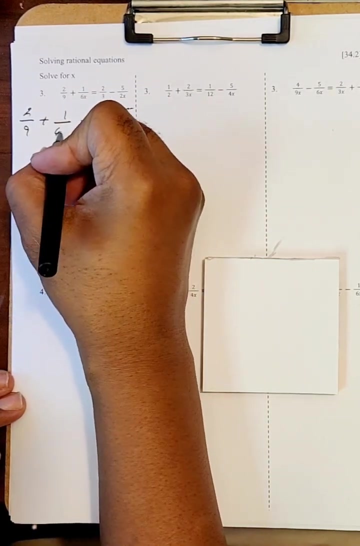 Solving Rational Equations. First, we want to find a common denominator for all our denominators. So let's write our problem here: Fraction plus fraction equals fraction minus fraction, And we have a 2,, a 1,, a 2, and a 5 as numerators. We have a 9,, a 6x, a 3, and a 2x. 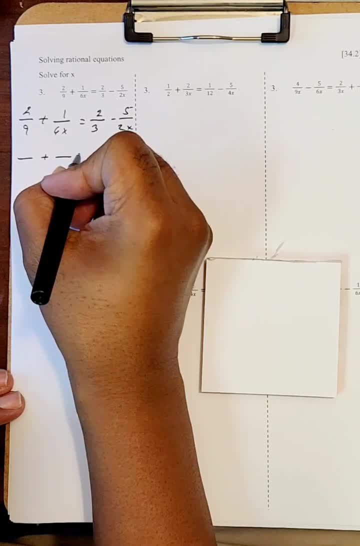 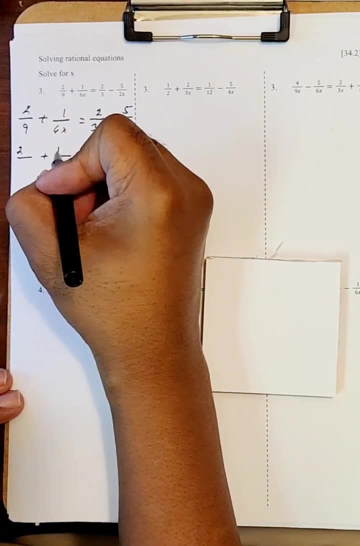 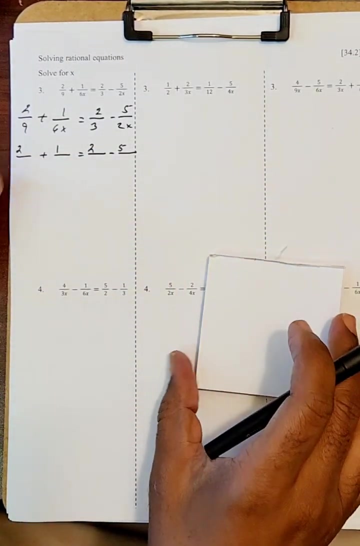 Okay, so we'll begin the process of finding new denominators Now. the old denominators, old numerators, are 1,- sorry- 2, 1,, 2, and 5.. We'll put those there Now. our denominators, as far as the numbers are concerned, are 9,, 6,, 3, and 2.. 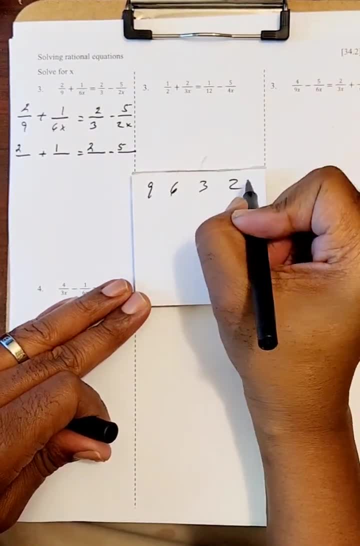 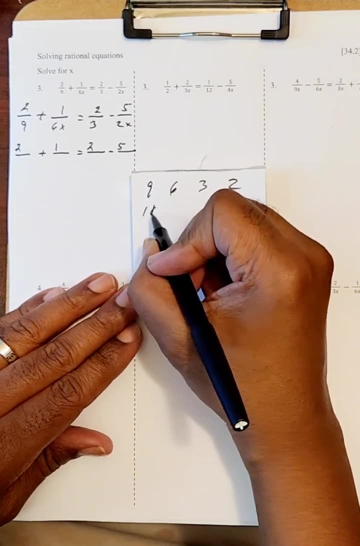 So 9,, 6,, 3, and 2.. And we want to find the least common multiple. So let's go with 9 here. Let's go with 9,, 18,, 27, and 36.. We'll stop there. 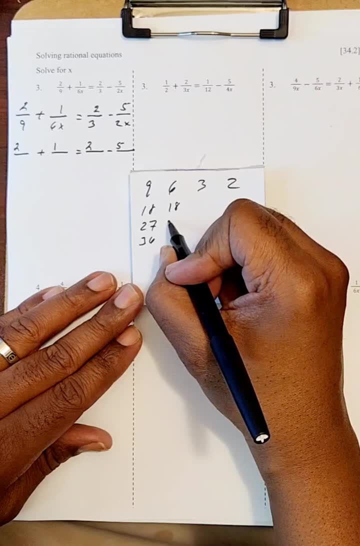 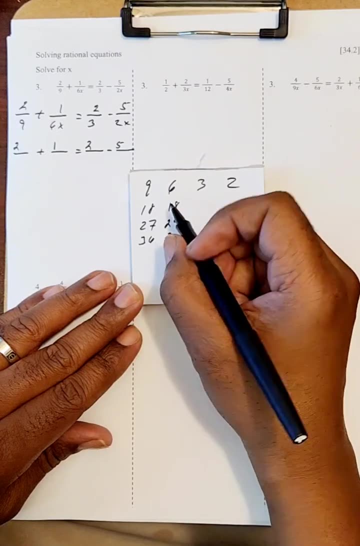 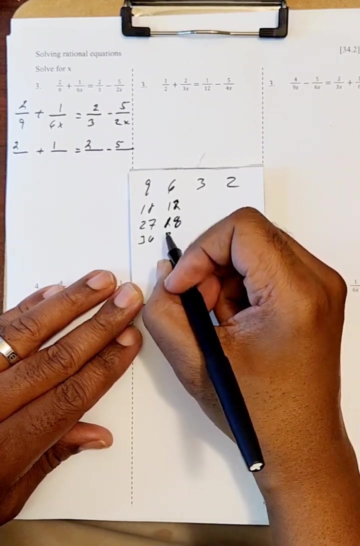 6, and then there's 18,, and then there's 24,, and then there's 30.. Let's see, I skipped 12.. Sorry guys, There's 12, and then there's 18, and then there's 24.. We'll stop there. 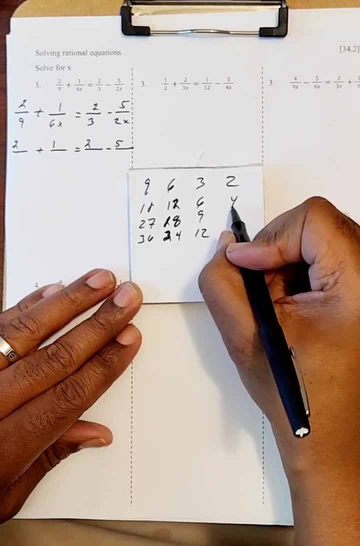 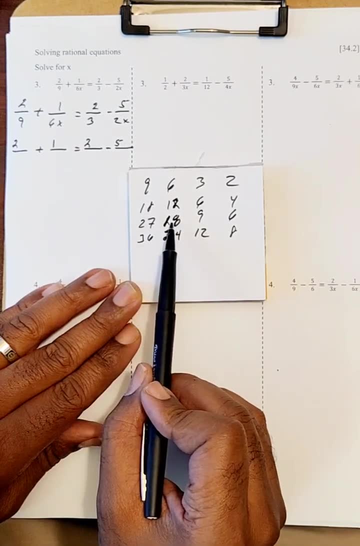 3, 6,, 9,, 12, and 2 is 2, 4,, 6,, 8.. Okay, I'm seeing a little bit of a pattern. I'm starting to see 18 show up here, so twice here.